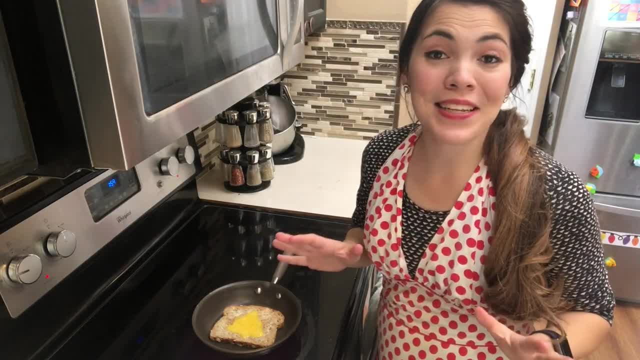 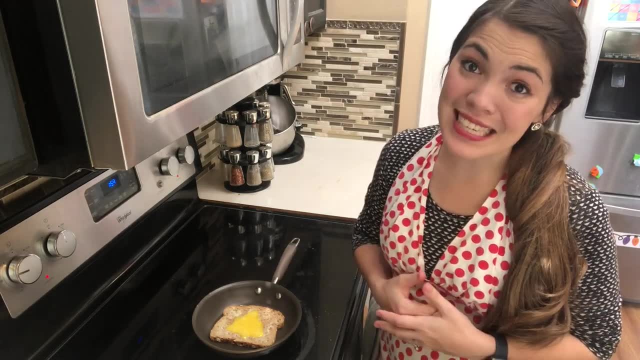 Today we're going to go scramble. I totally, totally forgot to mention the most important part of this video, and that is that all of these foods today are going to be healthy foods. It is so easy to fill this season with things that make your heart feel good. 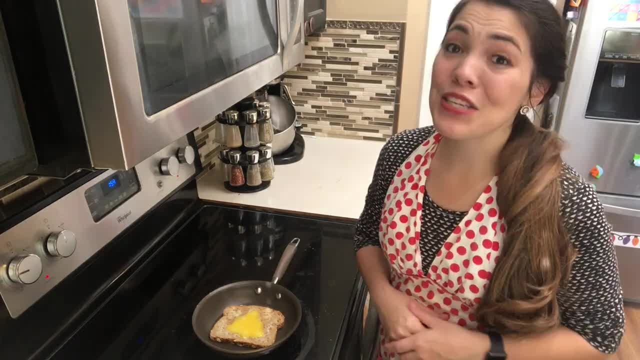 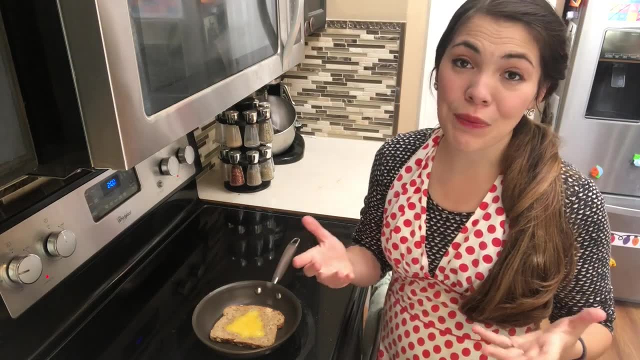 but they might not exactly make your whole body feel good. So, for yourself and especially for your whole family, we're sharing 10 fun Christmas-themed foods that you can share with your family that are healthy and will give your bodies more of the things that it needs. 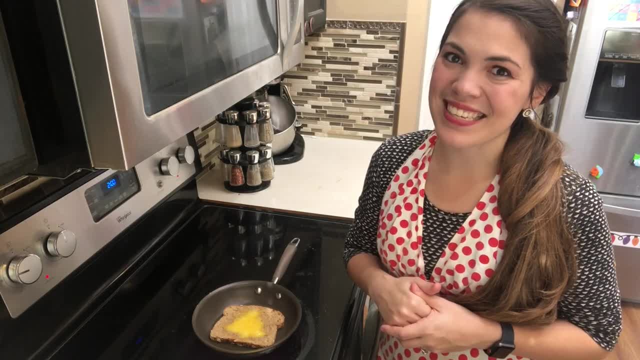 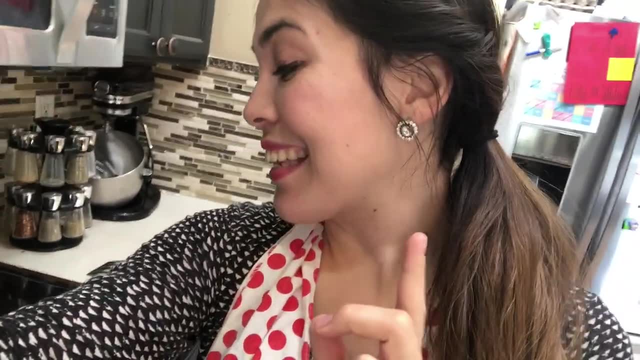 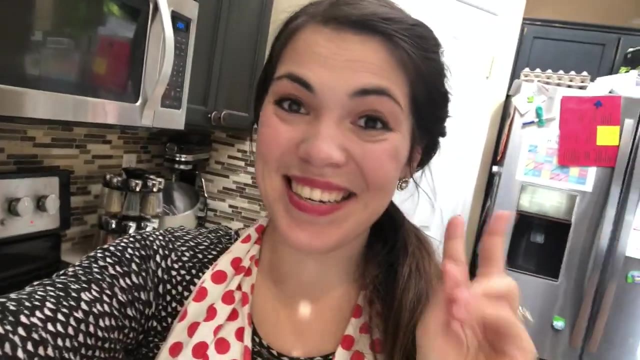 maybe to compensate for all the extra things that your body is getting this season. Okay, that might not have been exactly ready to flip yet. It is a little juicy and spilled over, but it's okay. It still looks like a Christmas tree and it's still fun. Let's move on to number. 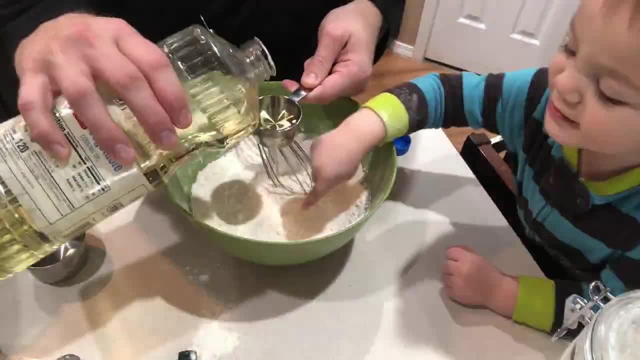 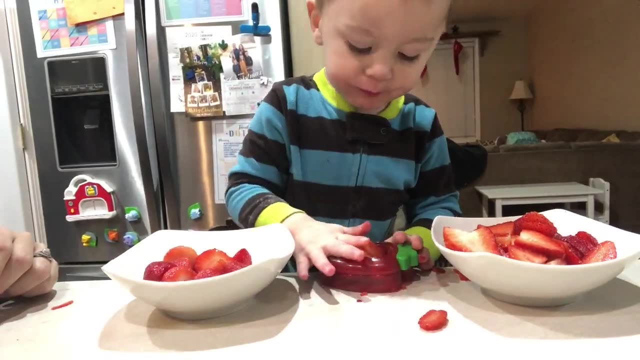 two. Another super, super fun breakfast is Santa pancakes. We're making up a normal batch of pancakes, but we're going to use strawberries to top Santa's hat and personally. we're going to add a little bit of whipped cream for his beard and his hair. We're going to add a little bit of. 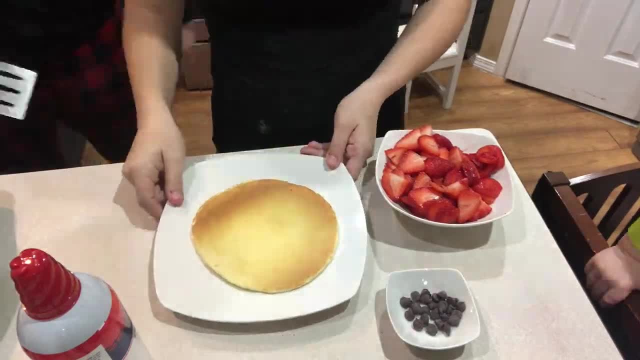 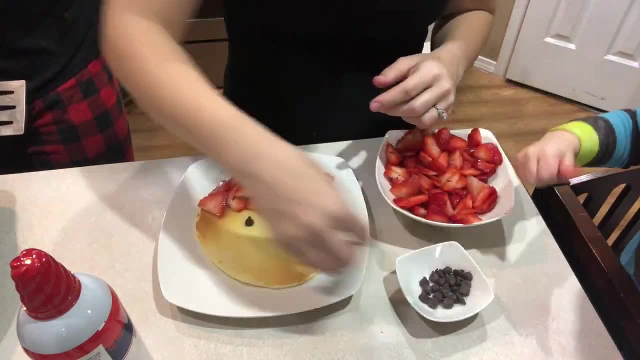 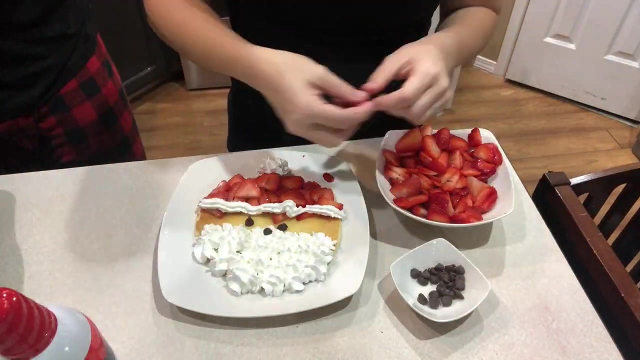 whipped cream and the fluff on the hat, but if you want to make yours extra healthy, you can sub out the whipped cream for bananas. This is a super fun Santa-themed fluffy breakfast that can be nearly 100% healthy if you want it. I do have to admit we also used chocolate chips for Santa's. 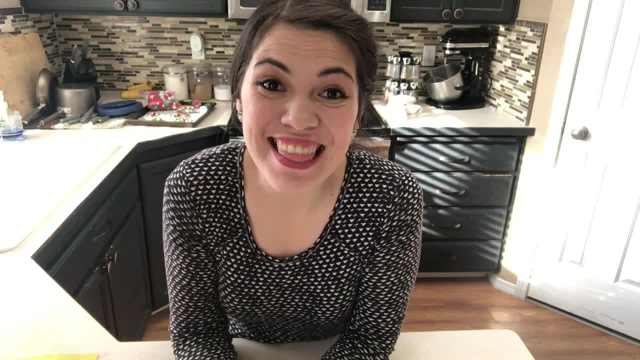 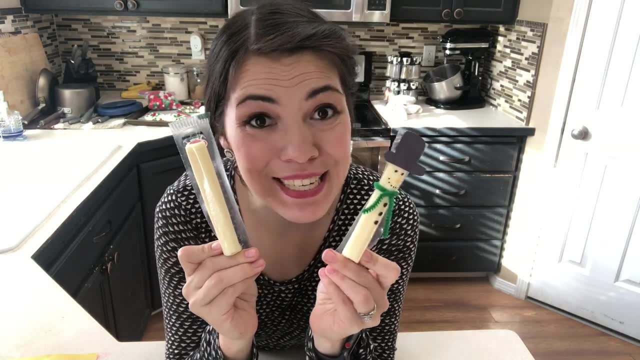 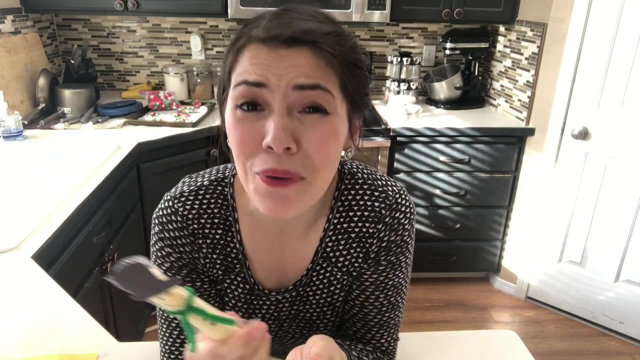 eyes as well. Next, we are going to be doing a Christmas-themed snack, turning this boring old Christmas into a Christmas-themed one. The one thing I love about these cheese sticks is that they are so fun, so easy and so portable. They make great snacks that you can actually prepare. 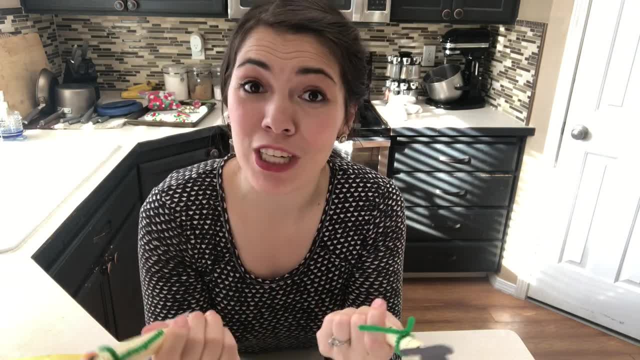 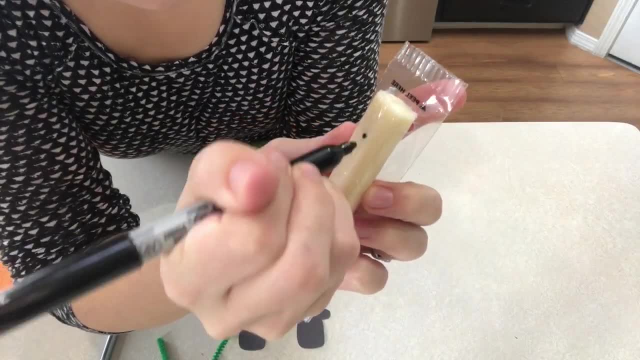 in advance and just throw in your fridge, or you can even send them to school with your child in their lunchbox so that they have a nice festive, healthy snack. Like I said, these guys are super simple. Use a Sharpie to draw on the eyes, the mouth and the buttons of your snowman, Then 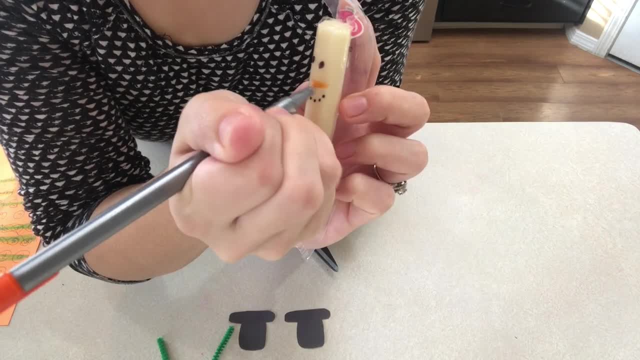 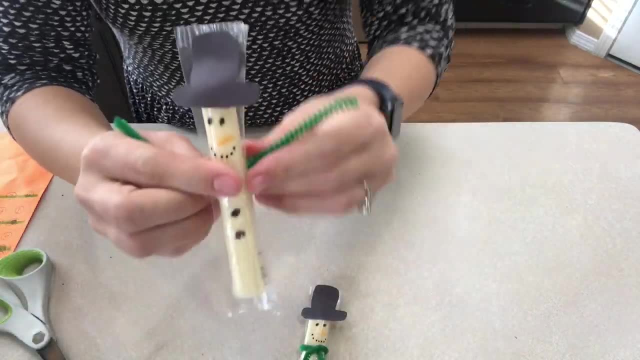 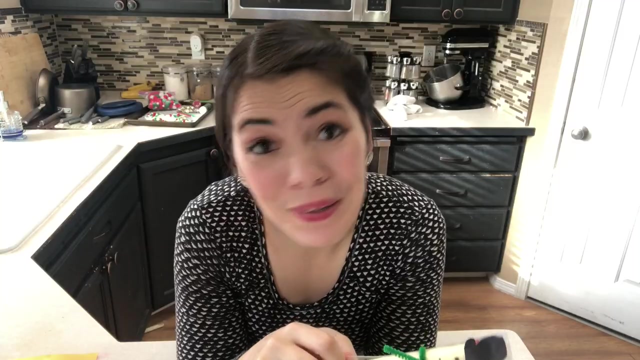 you'll need orange to draw on that iconic carrot nose. Don't forget the carrot nose. Then we simply used construction paper to cut out a hat and a pipe cleaner to add as a scarf. You could also use ribbon or yarn or really whatever you had lying around for that scarf. When you're all done, 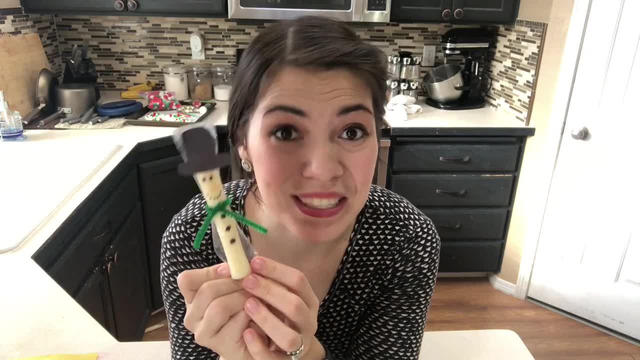 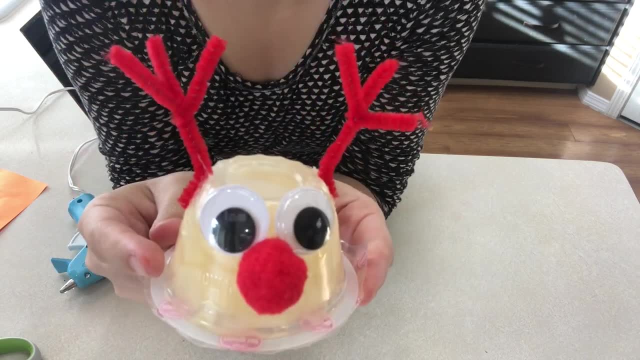 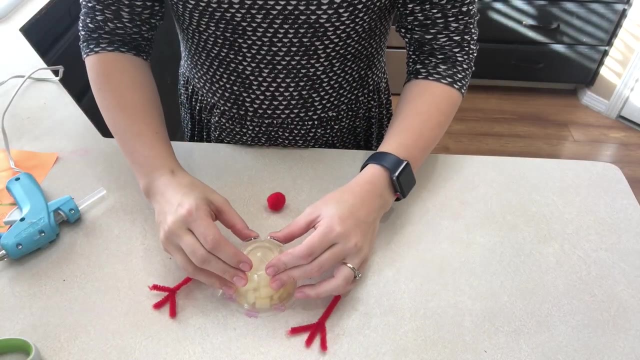 you'll end up with these irresistibly adorable little snowmen. Our next Christmas-themed snack is also a great snack that you can take on the road or pack with your school-age child to send to school, and these are reindeer-styled fruit cups. Now, this works with applesauce or diced. 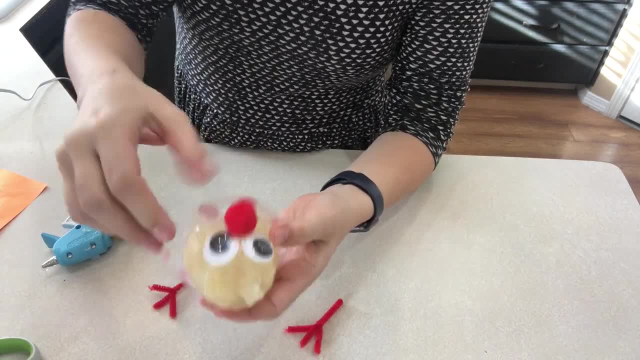 peaches, and it's a great snack to have with your family or friends. It's also a great snack to have with your family or friends. It's a great snack to have with your family or friends. It's a great snack for preaches. diced pears, mandarin oranges, Anything that comes in a bit of a cup, It's not. 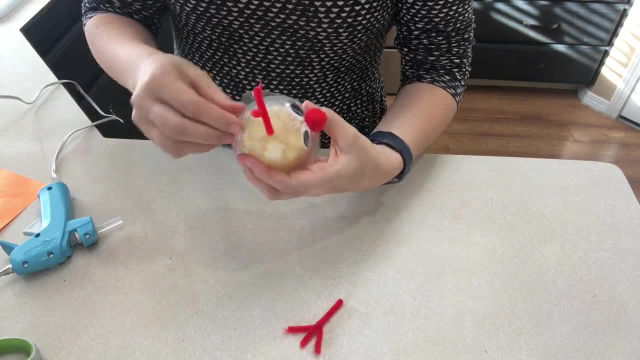 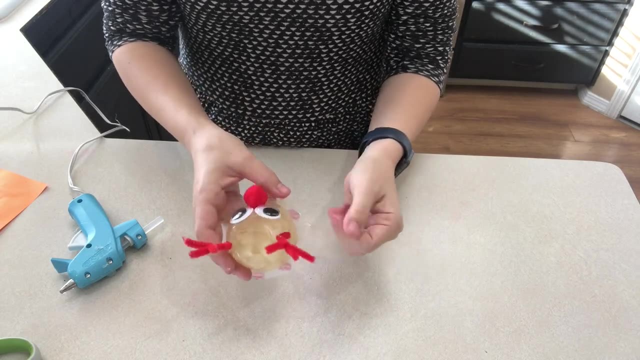 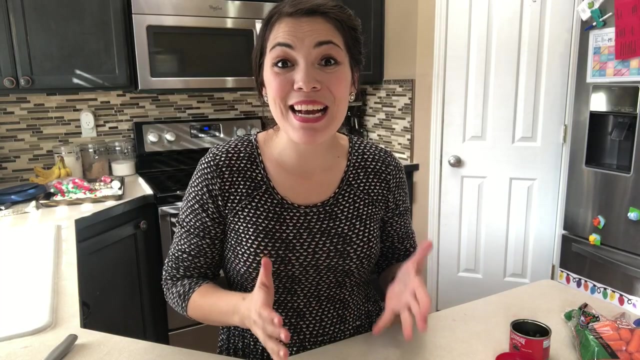 so healthy, but you could also do it on pudding. That works great too. Use pipe cleaners as antlers. googly eyes as well the eyes and a nice red pompom for the nose. Hot glue these reindeer accessories to your fruit cup for a nice Christmas snack. All right, now we are going to be making 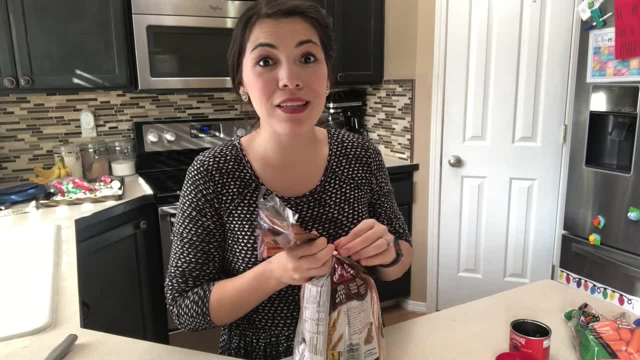 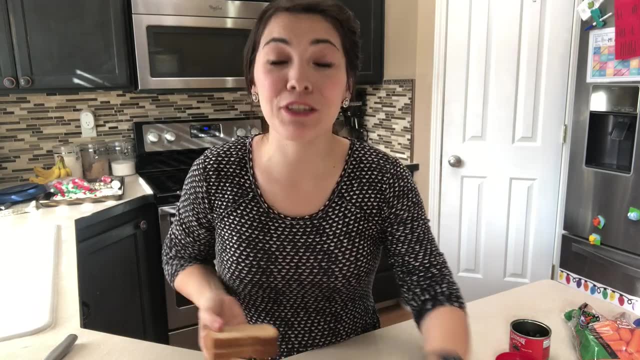 our way to lunch time. This is a great, simple lunch. It's something that you're probably already doing and just adding a little bit of fun. We're gonna start off by making your child their favorite sandwich. It could be peanut butter and jelly. 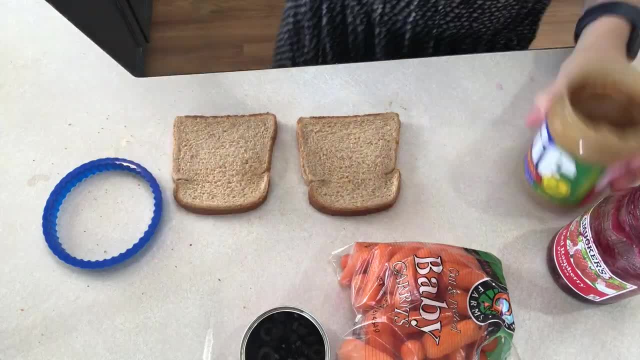 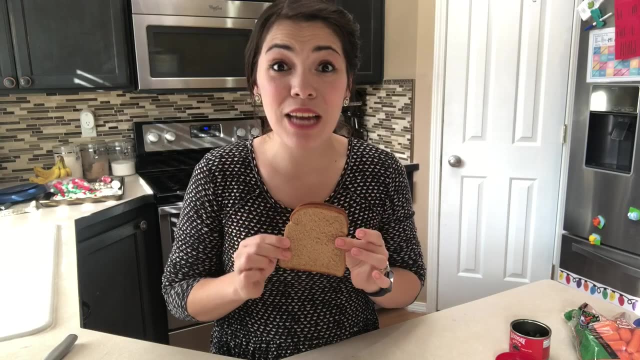 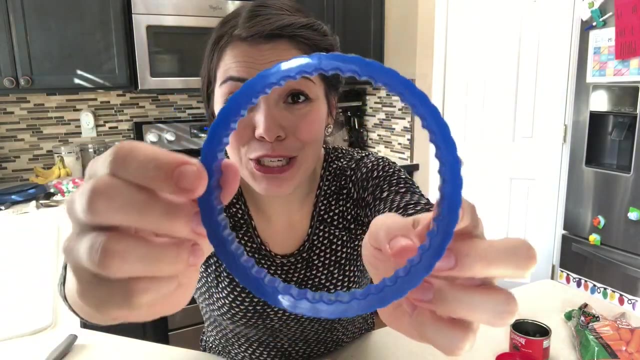 doesn't matter what it is, but just start by making their sandwich. After their sandwich is made, we're going to go ahead and use a large circle cookie cutter. Now ours actually happens to have ridges around it. I just thought it was cute. 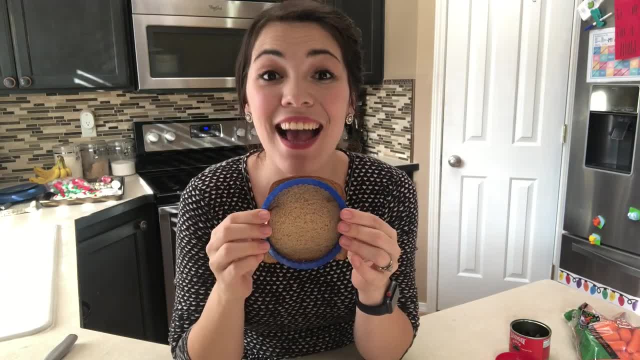 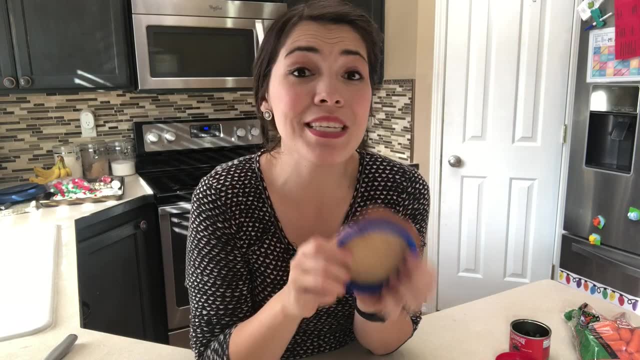 And we're gonna place it on top of our sandwich and cut out the shape. Spoiler alert: we are making a snowman with our sandwich today, But if you wanted to make a Christmas tree or a stocking or Santa Claus, you can use whatever cookie cutter. 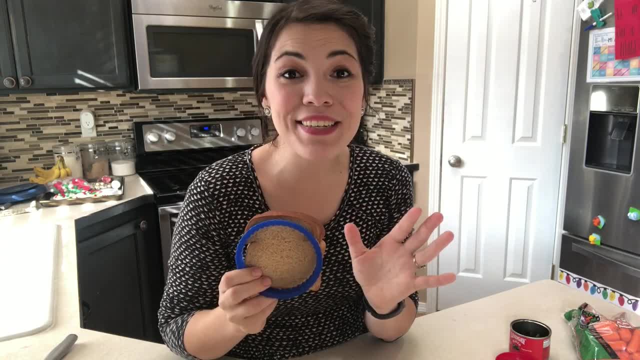 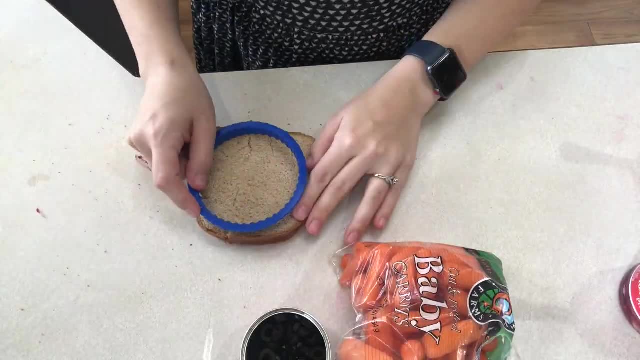 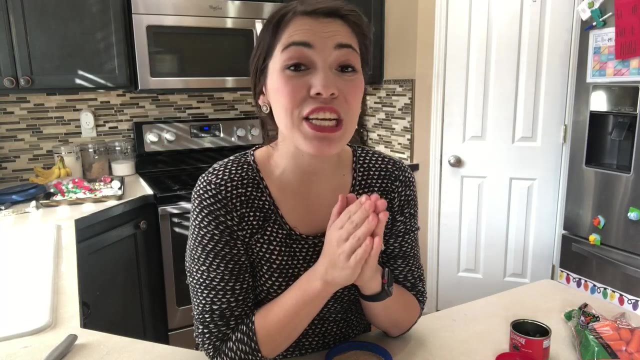 to make your sandwich more fun. I don't know what it is, but cookie cutter sandwiches are always a bigger hit at our house than plain old, normal ones. Let's go ahead and get that cut out. Okay, now that your sandwich is all cut out, we're gonna add the very simple things. 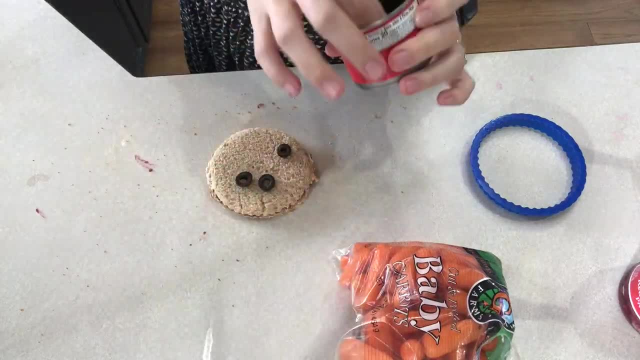 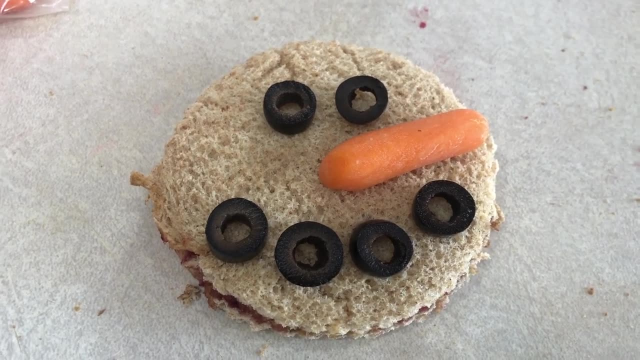 on the top to make it a snowman. Olives for the eyes, olives for the cold mouth and a carrot for the nose. So simple but so cute and inviting for your child to eat. Next to our lunch special, we are going to add some cheese trees. 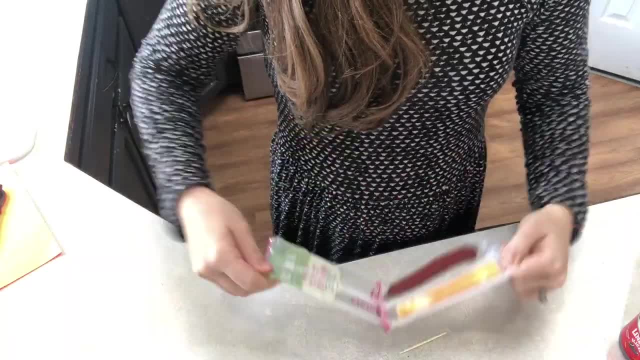 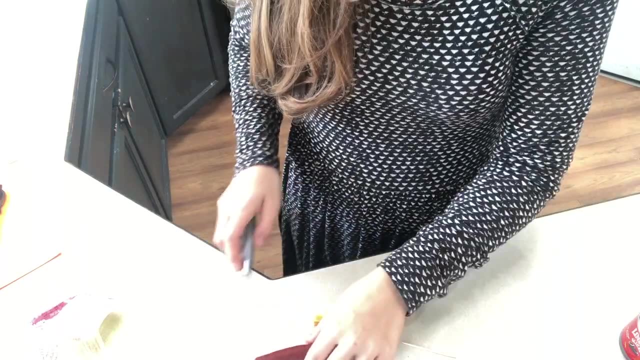 I actually never had purchased these before, but these little packs of cheese and meat- or in this case, ham- are not only fun and would make a good snack individually, but it's a quick way to add a good source of protein and dairy to your child's lunch. 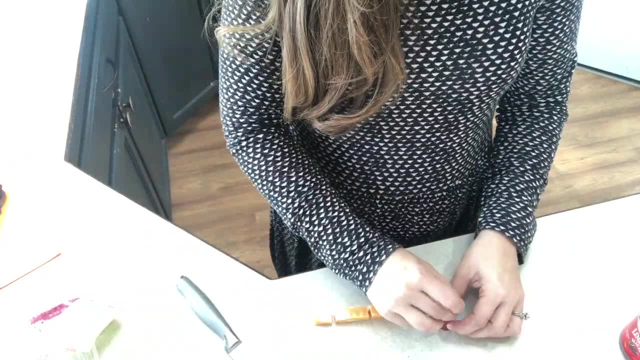 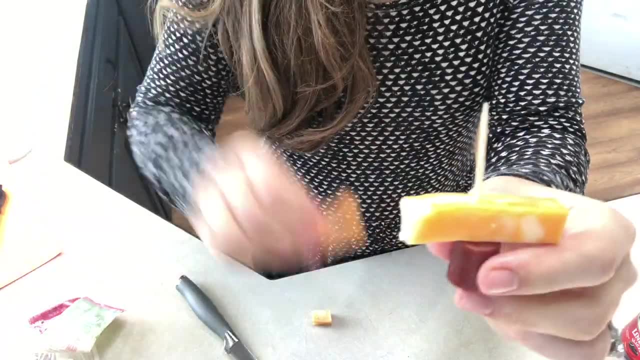 Cut both the meat stick and the cheese into different size slices: a large piece of cheese for the bottom, a medium piece of cheese for the middle and a small piece of cheese for the top, giving your cheese that tree effect, and stick them all on a toothpick. 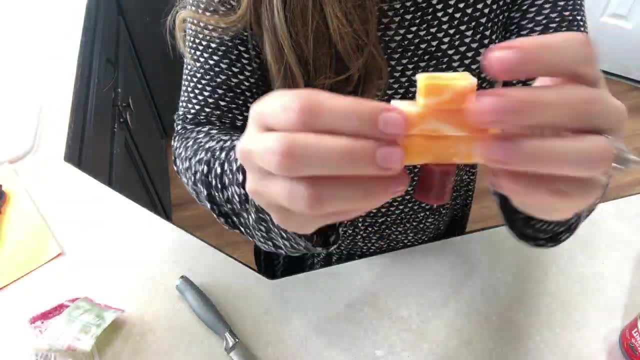 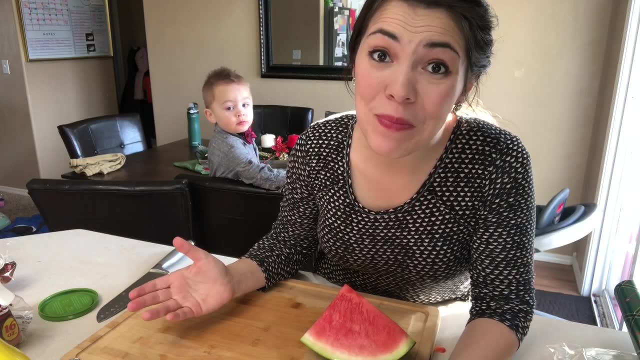 Now, if you have younger children, you might want to omit the toothpick and you could easily just lay it on their plate. The next one is super simple To add to our lunch. we are gonna make some watermelon Christmas tree. 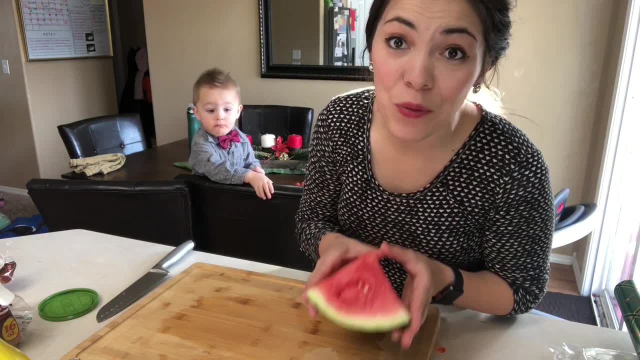 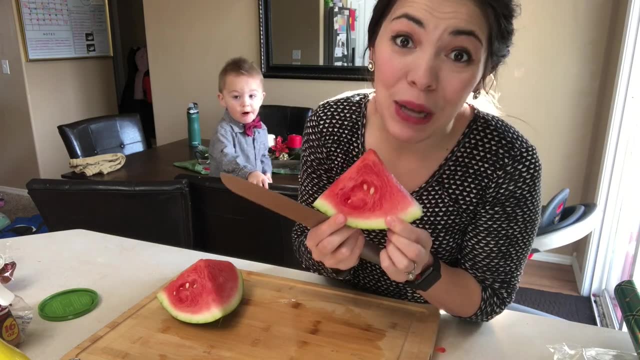 So you'll want to pre-slice your watermelon into a nice little triangle wedge and then slice your watermelon like you would if you were gonna slice it for a barbecue or something With your nice little triangle piece. now we're just gonna cut off parts of the stem. 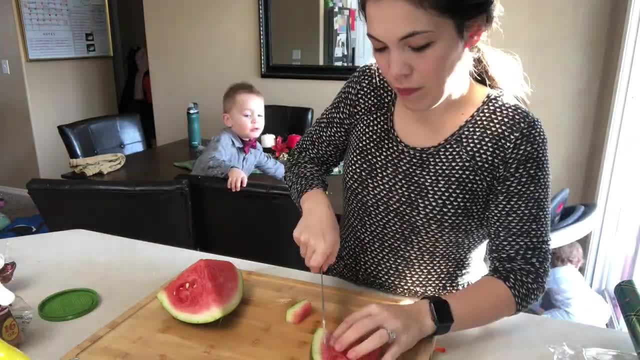 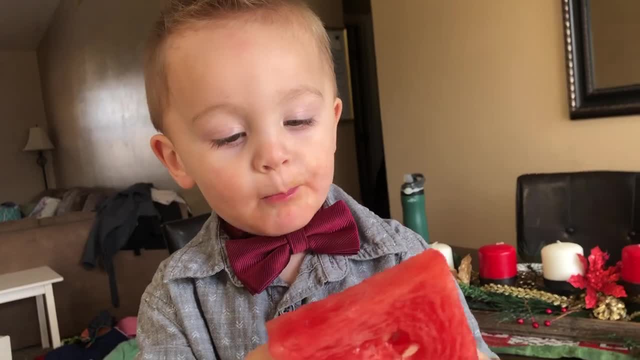 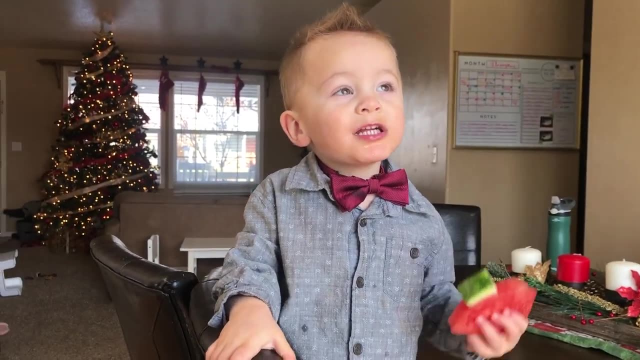 on the left and on the right. Mine's a little off-center this time, but look at how cute this little Christmas tree is. What do you got? I have watermelon this way too. I have watermelon this way too. How's your watermelon Christmas tree? 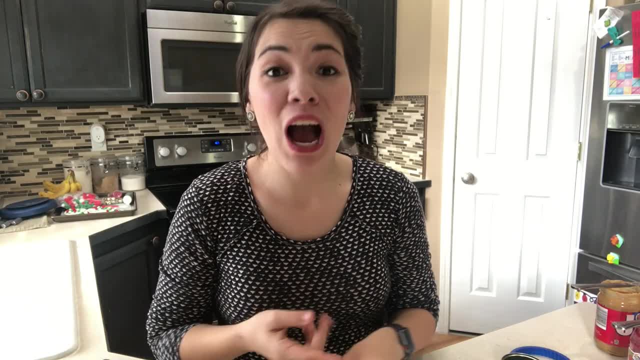 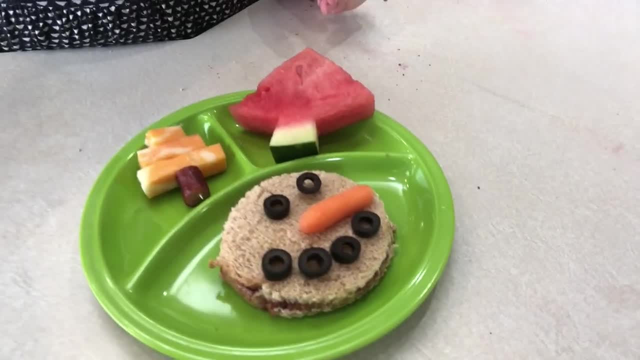 Yummy, Oh good, Now that we've got our snowman sandwich, our cheese tree and our watermelon tree, let's put them all together for our lunch today and see what we've got. Look at how cute this is. 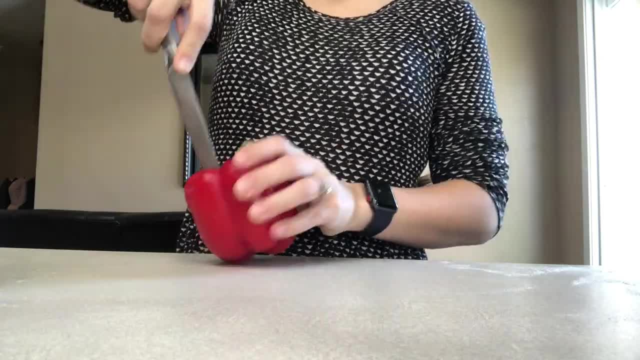 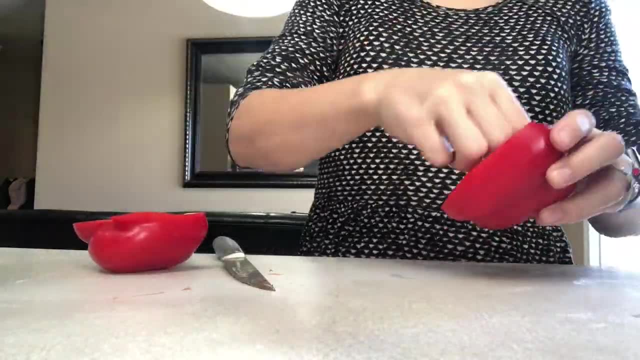 I think they're gonna love it. Our next Christmas, healthy food is going to be a snack. This one is so simple and it just shows how a little bit of creativity can go a long way. Slice some red bell peppers, Then using a Sharpie. 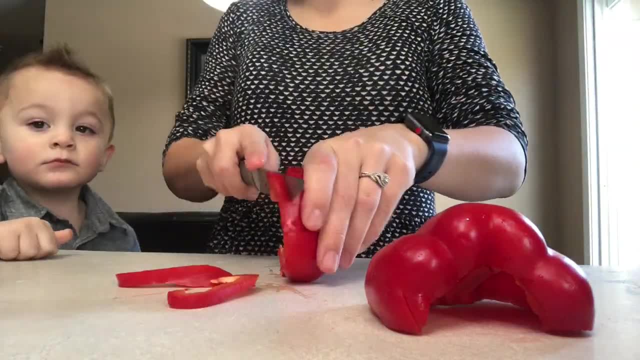 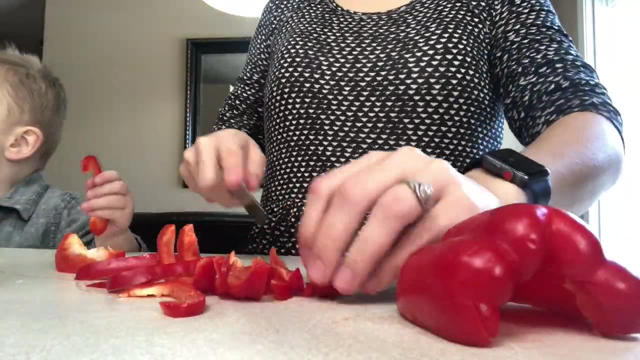 you can draw Santa's belt around the cup, preferably a cup that you don't mind throwing away. Add a little ranch to the bottom of your cup, if you desire, and stick those sliced red bell peppers right on top. It's a simple way to add a little bit of Christmas. 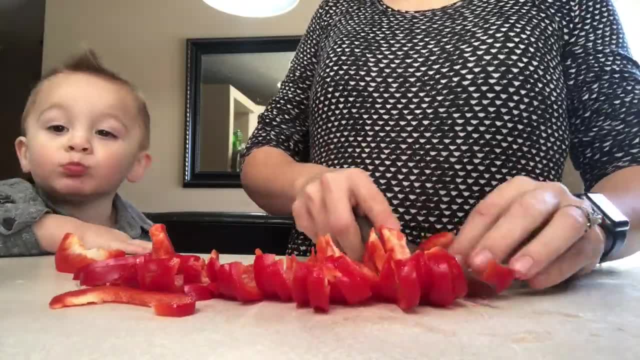 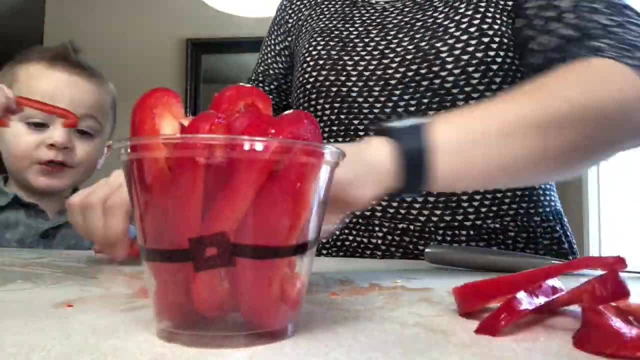 to your snack, while also sneaking in an extra serving of veggies. And if your kids are anything like mine, the crunch on peppers really just makes for a great snack. So dressing it up was just an added bonus. Mmm, What do you got bud? 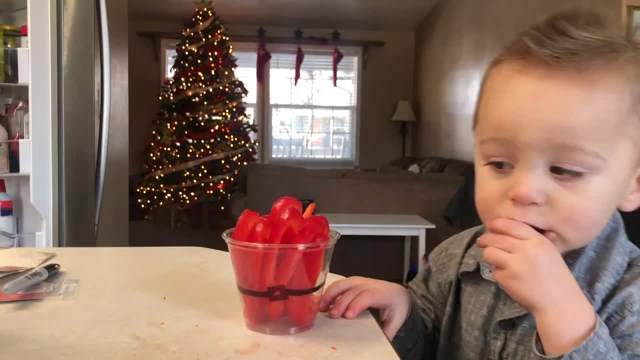 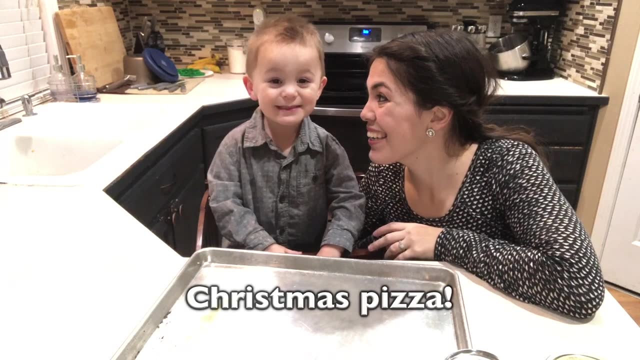 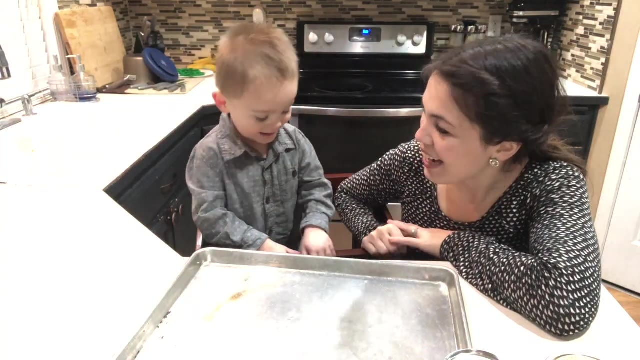 Puppets, Some peppers, Mmm crunchy red peppers. You're kind of goofy. There you go. What are we making? Christmas pizza. Say it again: Christmas pizza, Christmas pizza. Are you ready to make some pizza? Yeah, 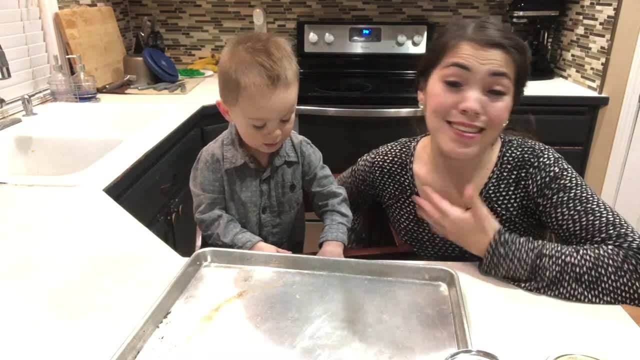 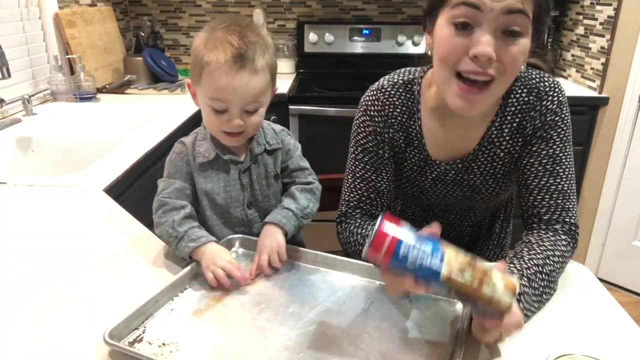 All right, This is a great one to do with your kids. It's not really one you prep in advance. more do together as a family. If you want to make some Christmas pizza, all right. Yeah, We just went ahead and bought some pre-made pizza crust. 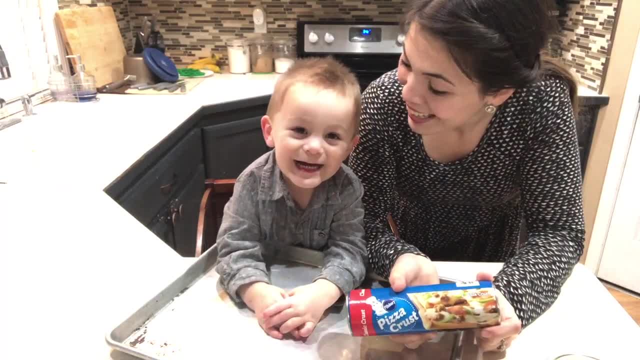 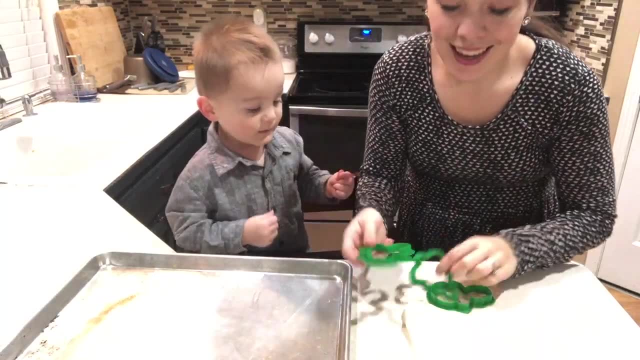 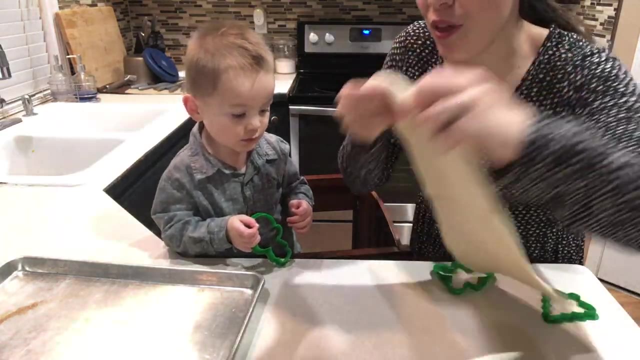 You can make your own if you'd like, but here we like to make things as easy as possible. When you get your crust all laid out, you will use some Christmas cookie cutters to cut out little mini pizzas. Now, we just did this with cookies the other day. 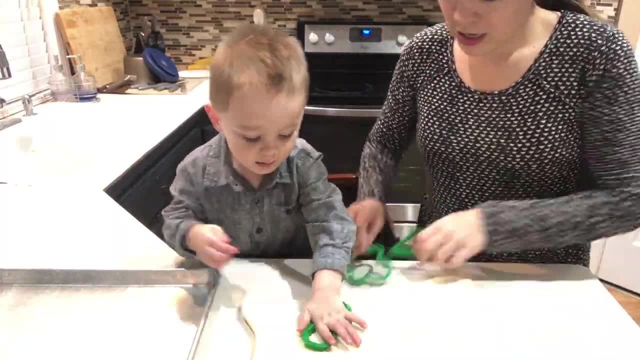 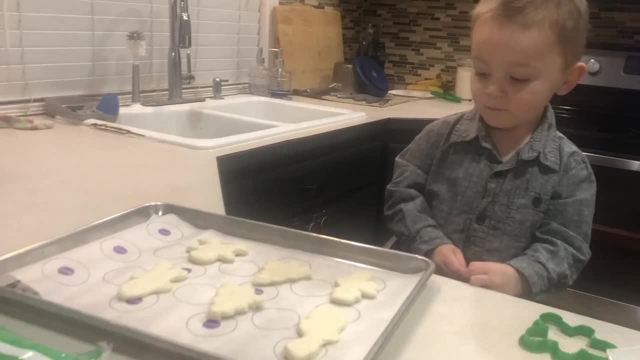 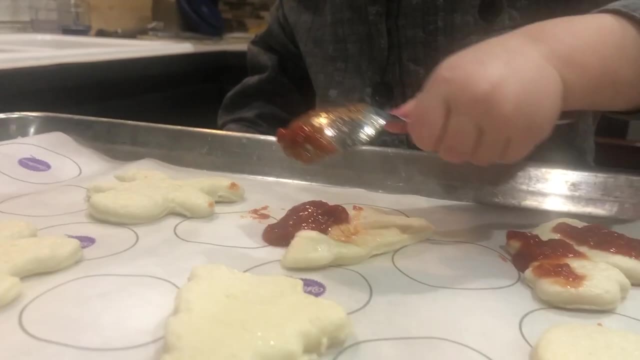 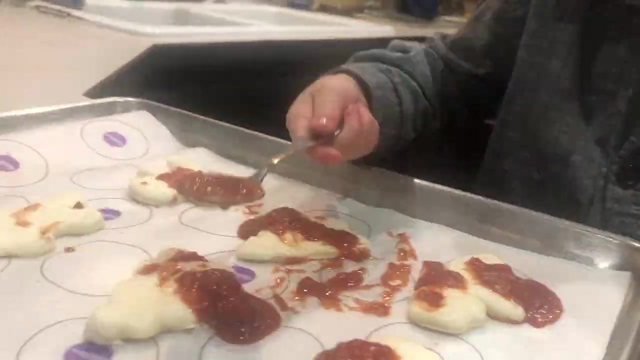 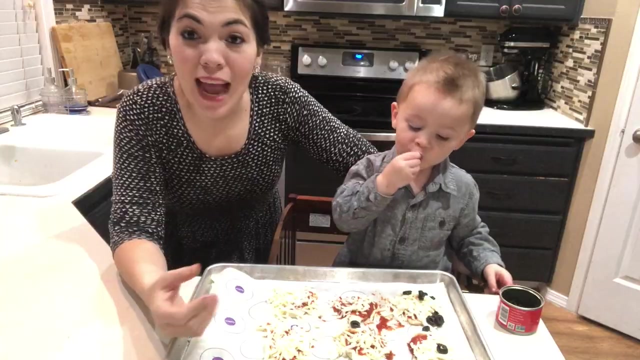 So Christian is a cookie cutter pro huh Yeah. Now we need to put the sauce on, Sauce on Mm-hmm Sauce on. After you get the bases of your pizzas all made up, go ahead and add all the toppings of your choosing. 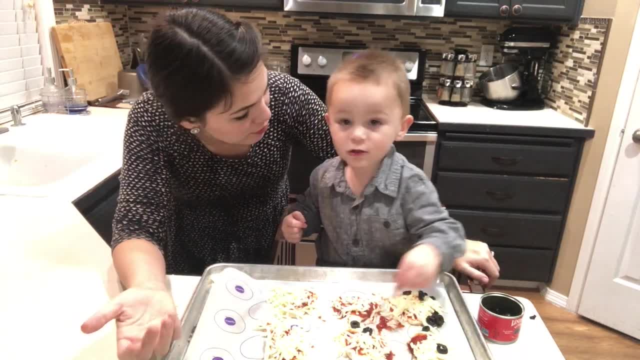 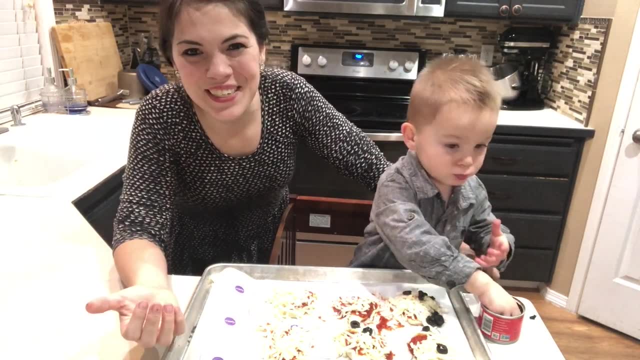 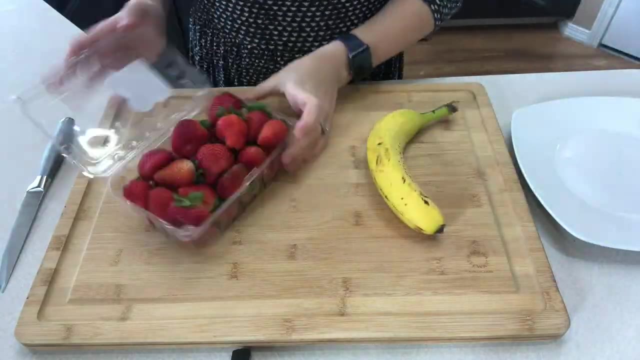 Cool. So Christian really likes olives. huh, Huh, Yeah. And so Christian's adding lots of olives to his tummy and maybe some to the pizza too. Our last healthy Christmas snack for your family would work great with breakfast. 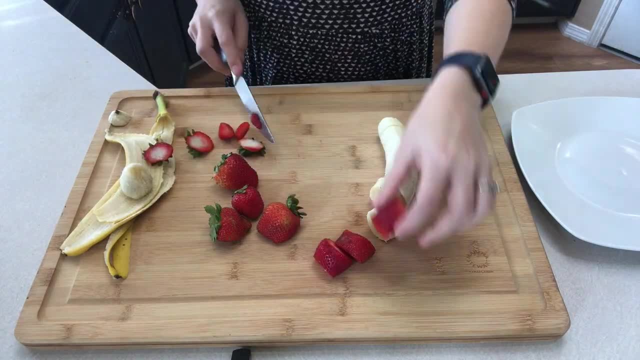 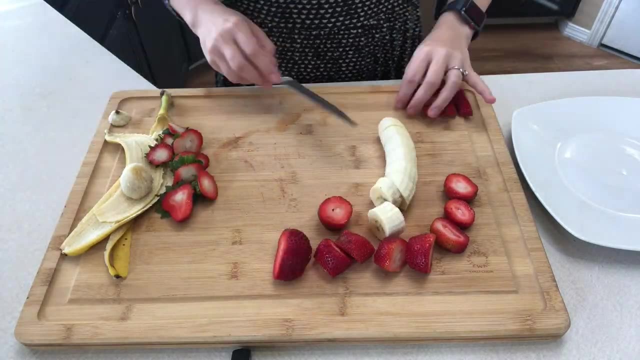 It would work great as an after-school snack. And this is our Fruity Candy Cane. Cut thick slices of strawberries and bananas and alternate them into a candy cane pattern: One banana, one strawberry, banana, strawberry, banana, strawberry. 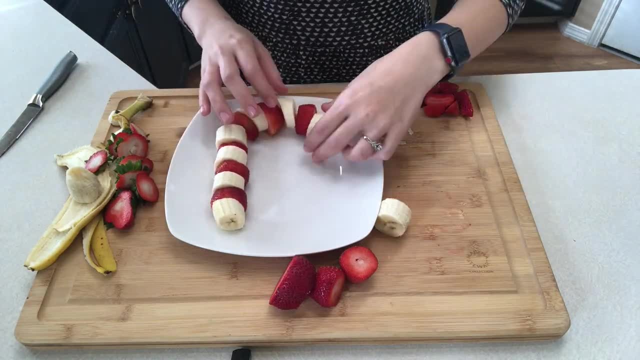 and so on, making your candy cane as large or as small as you want. It's 100% fruit and 100% delicious. All right, folks. Thanks so much for joining us today. We hope you enjoy these ideas of things that you can share with your family. 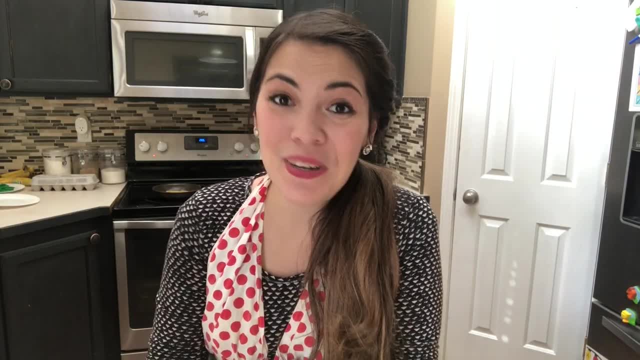 to help give their bodies more of the nutrients and the healthier things that they need during this Christmas season. I personally know that when I just mix it up a little bit it gets my kids excited about eating And you know they're going to love it.